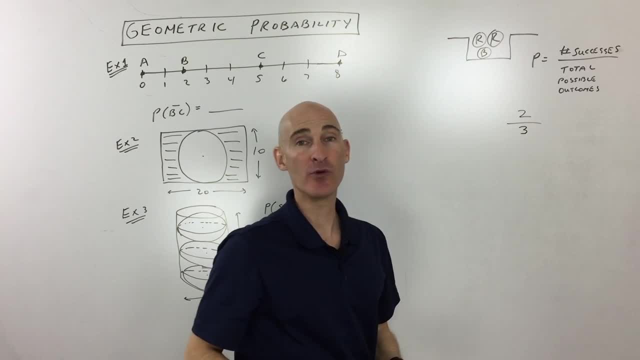 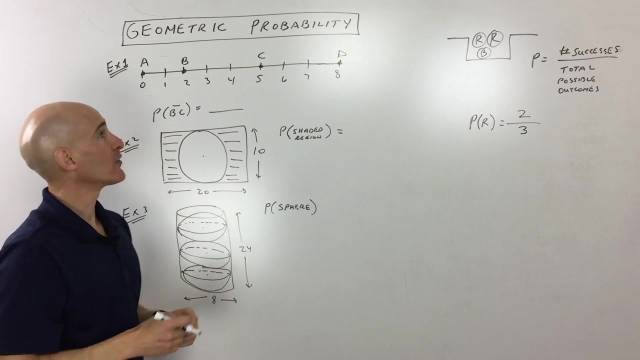 out of a total of three possible marbles. So the probability would be two-thirds of picking a red marble And you could write that as P of R, like the probability of a red marble. So let's get into some other examples here. So the first one: you can see we've got a line segment here. Okay, we've got some points on the line segment A, B, C, D. But it's asking us what's the probability that if we pick a point at random on this line segment- okay, let's say I'm blindfolded and I just pick a point- what's the probability that we lie? 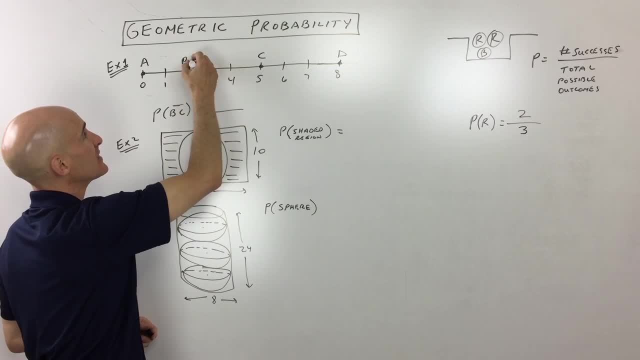 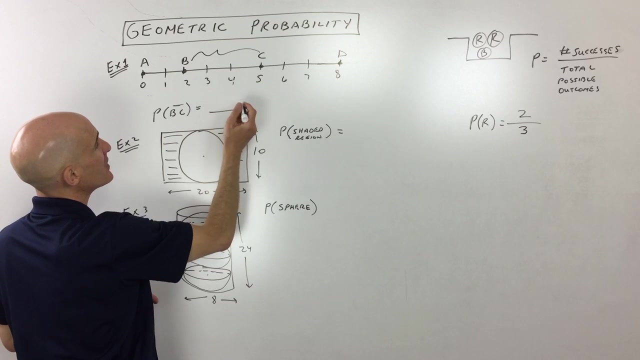 on this line segment, We pick a point that lies somewhere in between B and C. So right here. Well now, in this problem, what we're thinking about is the length of success divided by the total length. Okay, whereas over here we're counting the number of successes out of the total possible, Here we're considering the length of success, meaning the length that we want out of the total length. So in this case, you can see, it's one, two, three, Okay. so three units, okay, divided by a total length of. you can see. 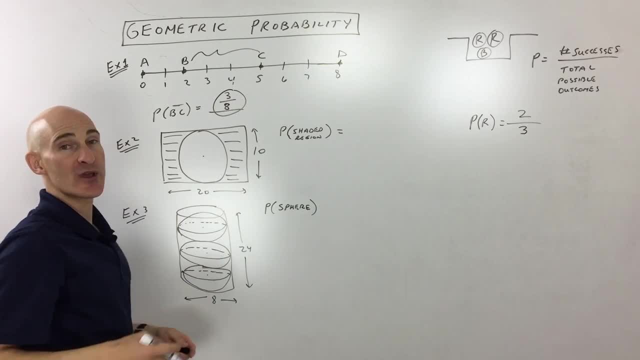 eight units. So our probability is going to be three eighths And you can write probability as a fraction or a decimal, Or if it says what's the percent chance, then you could convert it into a percentage. But probability in general is between zero and one. zero meaning no chance, one meaning 100% chance of success. Now example two. now we're moving from one dimension to two dimensions. we're talking about area And it's asking us what's the probability that you pick a point at random inside of this rectangle that it lies on the line segment. 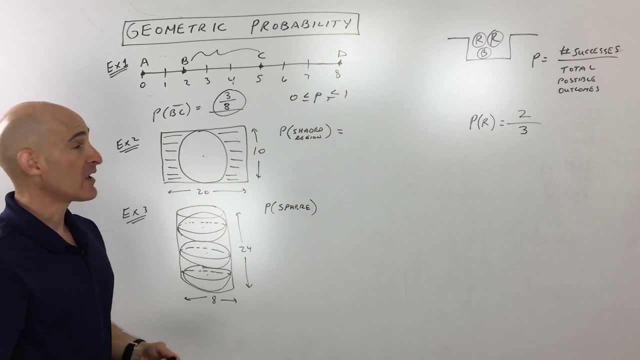 It lies in the shaded region, okay, outside of the circle. Okay. so again, what we want to think about is: what do we want? Well, we want the area of success. okay, the area of success, which is the shaded area divided by the total area. Okay, well, let's talk about this area of success. So, to get this shaded region, we're going to take the total area, which is 10 times 20, that's 200 minus we're going to subtract off the circle. Well, you can see that the diameter of the circle is 10, which means that the radius of the circle is 10.. 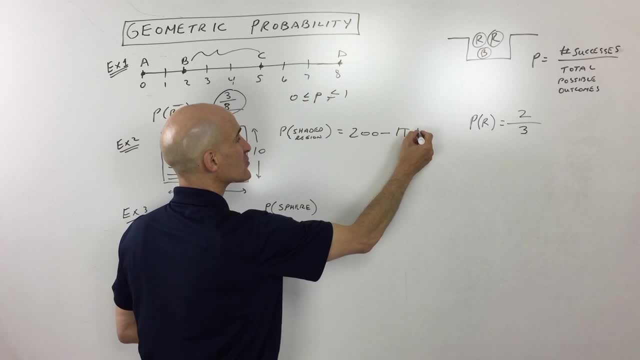 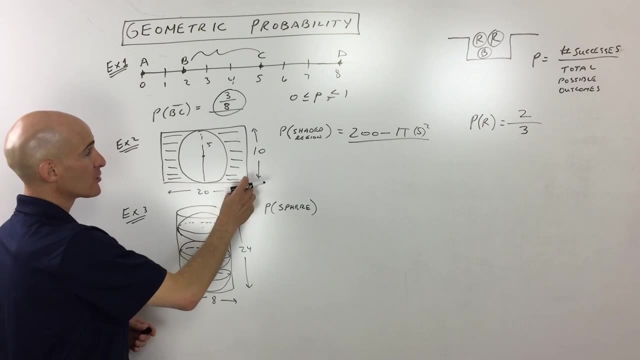 is going to be 5, which means we're subtracting pi r squared, which is pi times 5 squared. so that gives us the shaded region. now we're going to divide by the total area, which is the rectangle, 20 times 10, which is 200. so let's go to the calculator, let's see what, approximately what. 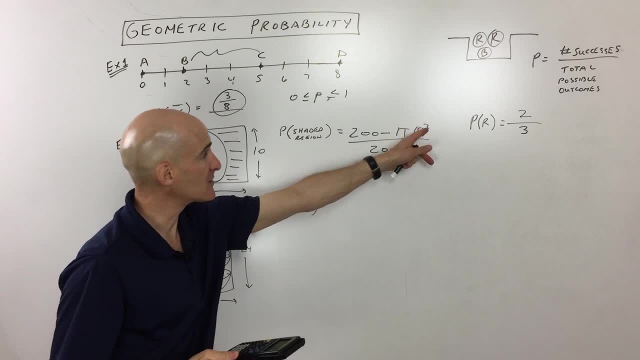 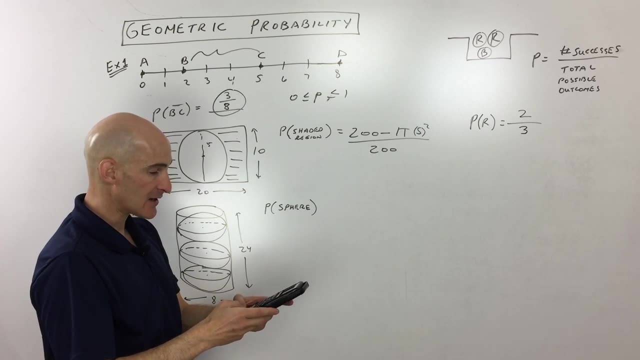 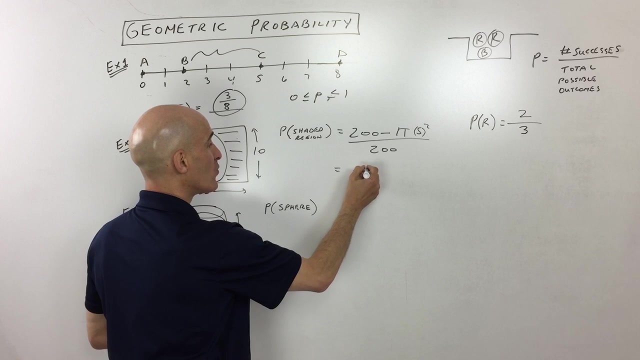 that comes out to we've got 200 minus 5. squared is 25 times pi. so 25 pi, let's see here, it's 121 approximately divided by 200. so it's coming out to about 0.61, or in other words about a 61 percent. 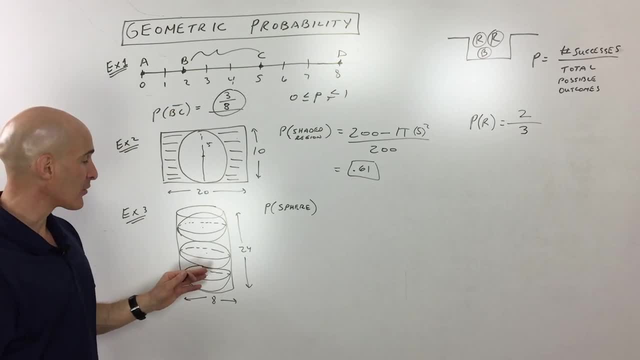 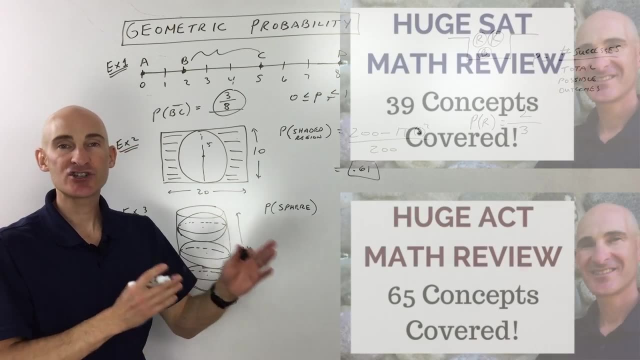 chance, but the probability is 0.61. now the third example. before i get into that one in three dimensions, i just want to mention that if you're preparing for the act or the sat, check out my huge act math review video course and my huge sat math review video course. we go through a lot of 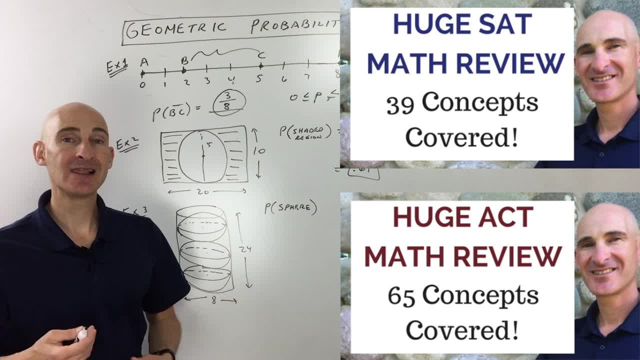 examples together, a lot of formulas, a lot of things that you would likely see on the internet, and i'll show you how to do that in a minute. so let's go ahead and get started examine how to approach those types of problems. so check out some of the free previews that are: 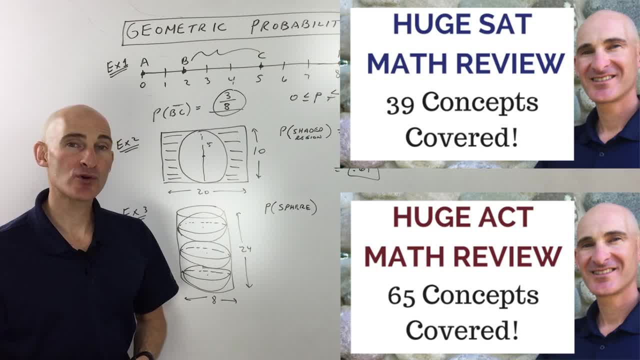 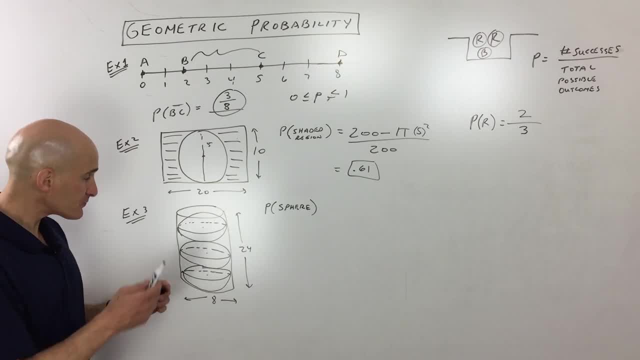 available, see if it's right for you. a lot of students have taken those courses and benefited. they said that they've improved their overall scores, so check that out and let's get into this. example three, though. if you want to talk about the volume now, okay, we're talking about the volume of 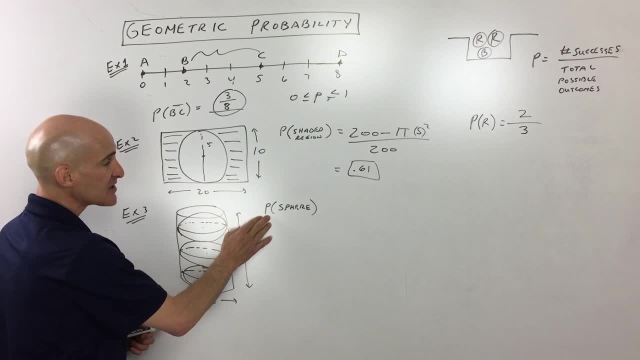 success divided by the total volume. in this case, it's asking us what's the probability that, if we we're talking about the volume of success, we're talking about the volume of one of these spheres times three, since there's three of them. okay, so it's kind of like tennis balls inside of a. 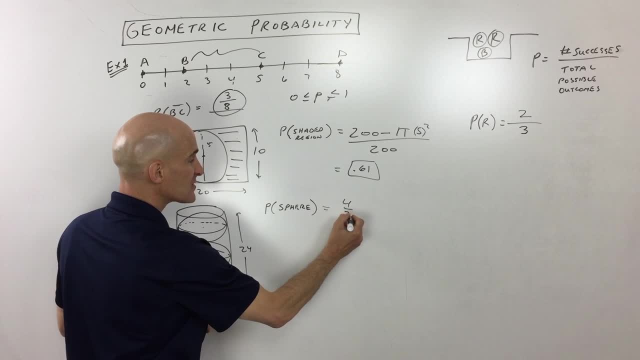 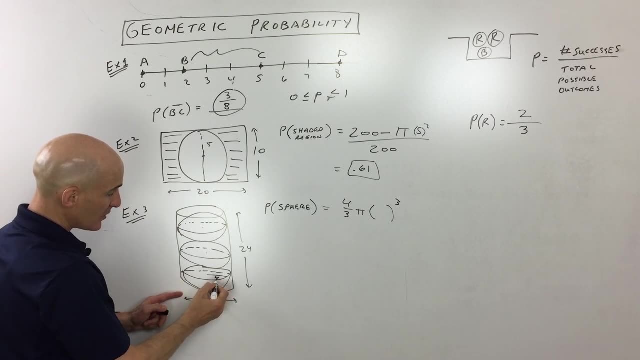 you know a cylinder right. well, let's see. the formula for volume of a sphere is four thirds pi r cubed. the diameter is eight. so that means that the radius of one of these spheres is four. so this is four thirds pi times four cubed. but remember, we have four thirds of a sphere.